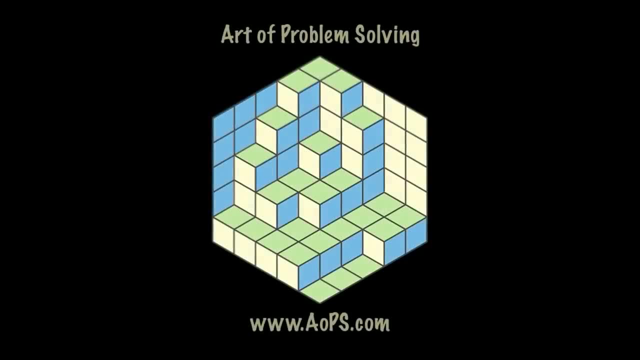 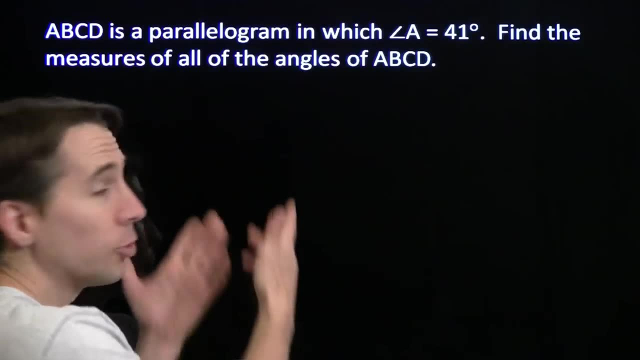 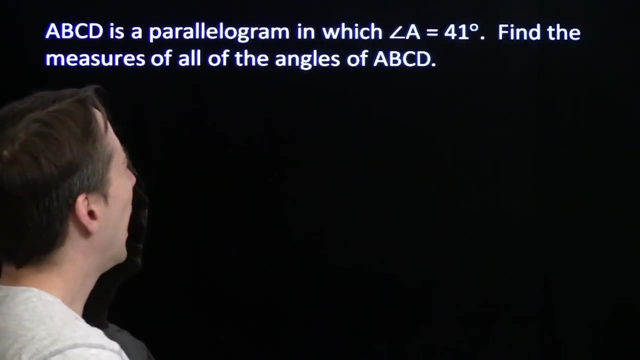 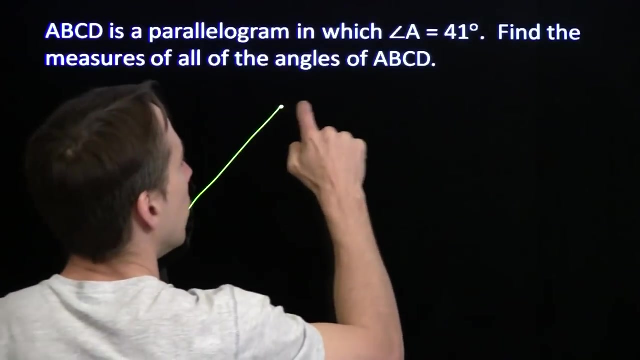 In this problem. we have a parallelogram, We're given one of the angles and we have to find all the other angle measures. How can one angle be enough? Well, our first step in a wordy geometry problem is to draw a picture. So go ahead and draw a diagram, draw a parallelogram. 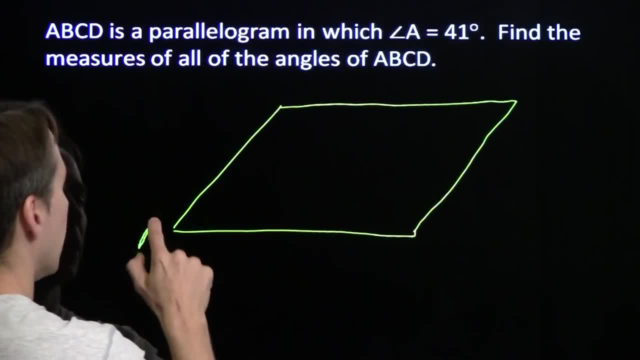 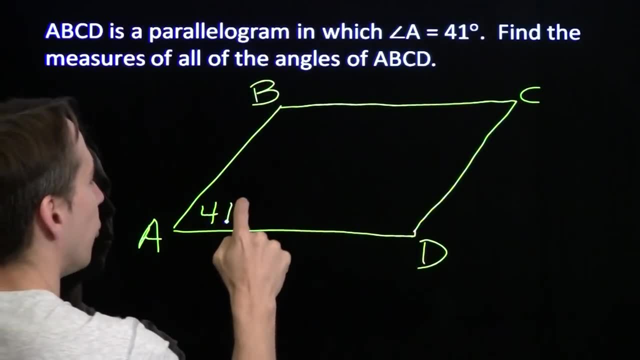 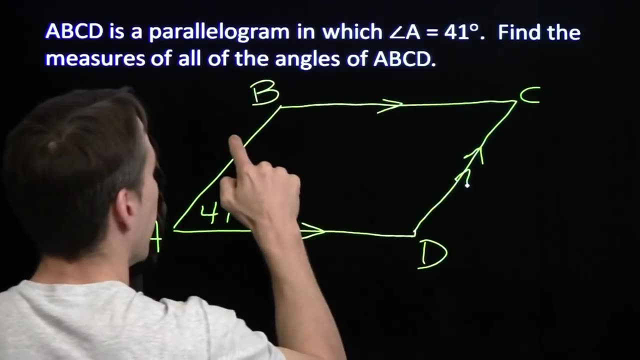 It means the opposite sides are parallel. Go ahead and label everything: A, B, C, D, And we know that angle A is 41 degrees And we know it's a parallelogram, so the opposite sides are parallel. We'll go ahead and mark that Because these two sides are parallel. 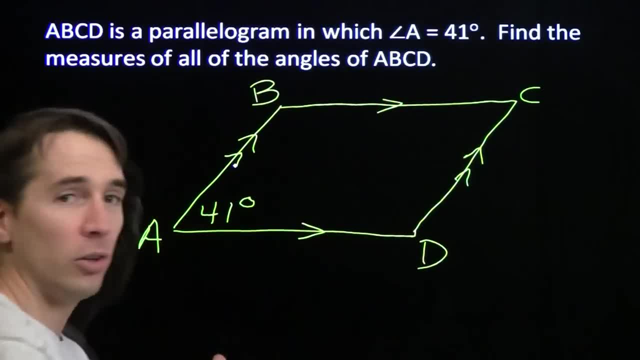 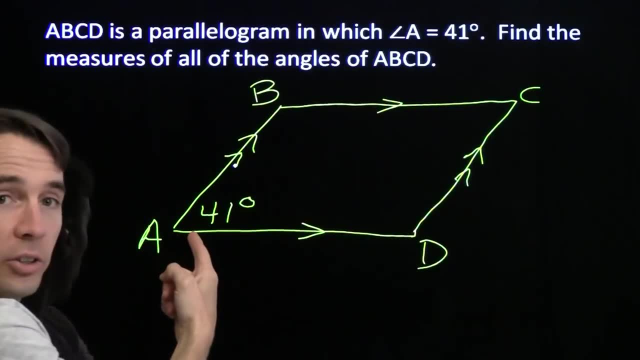 we can find this angle, We know this angle, this angle plus this angle, angle A plus angle D has to equal 180 degrees, Because these two sides are parallel. So angle D is just 180 minus 41 is 139 degrees And 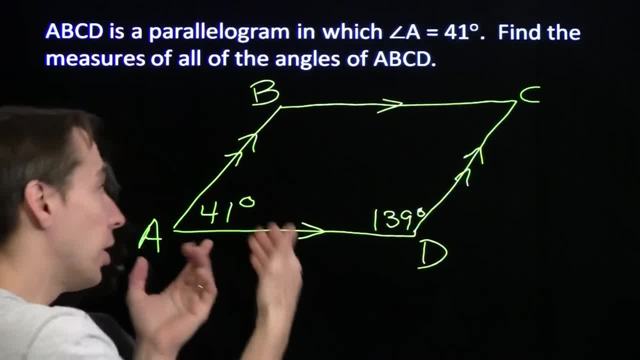 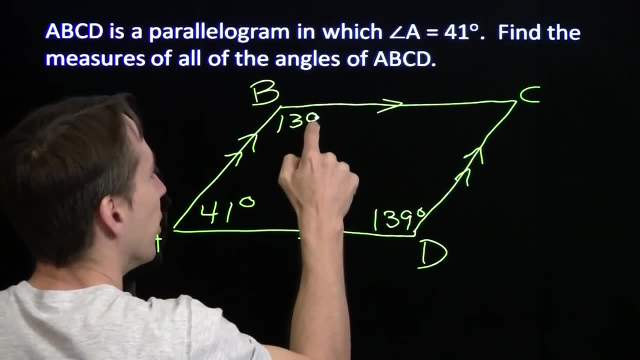 we can do the same thing up here. B, C and A, D are parallel, so these two angles, angle A and angle B, have to add up to 180.. So angle B is 180 minus 41 as well 139 degrees Then. 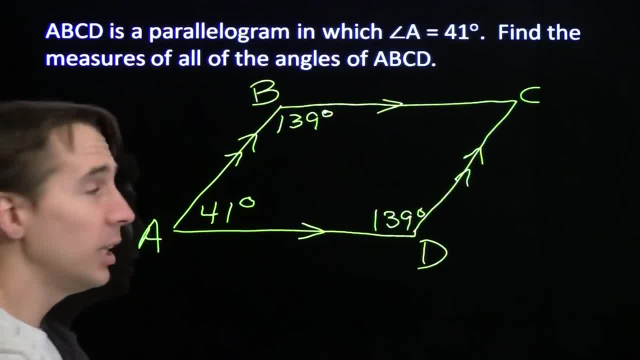 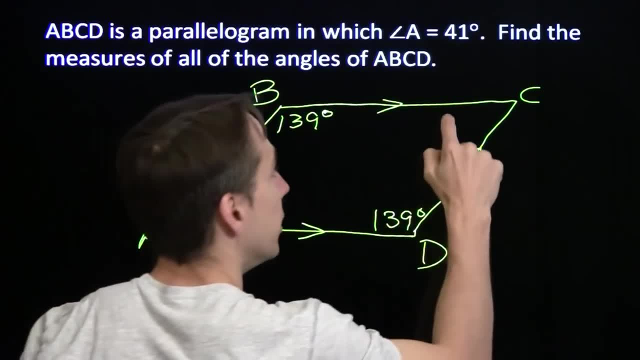 out here for angle C. well, once again we can use A B and C D. These two sides are parallel. These two have to add up to 180.. That angle is 180 minus 139, 41 degrees. Now check that. 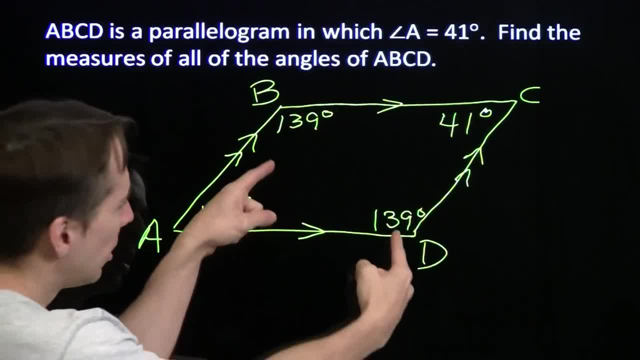 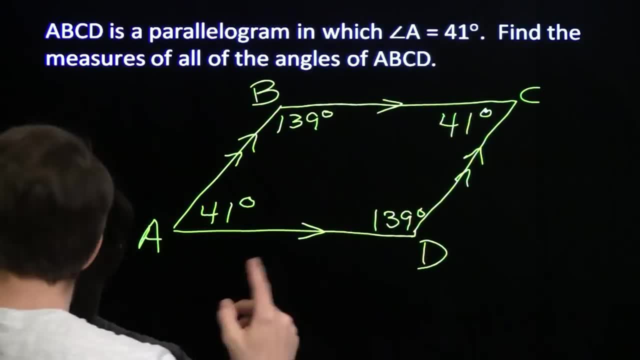 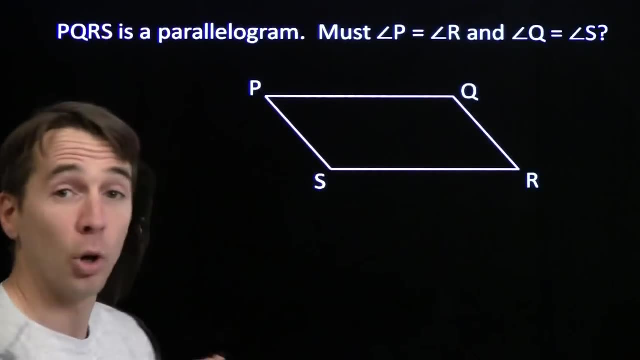 out. These two angles are equal. These two angles are equal. Will that always happen with the parallelogram or is there just something special about 41?? Let's check this out. Got a parallelogram and we want to discover whether or not these two opposite angles are always. 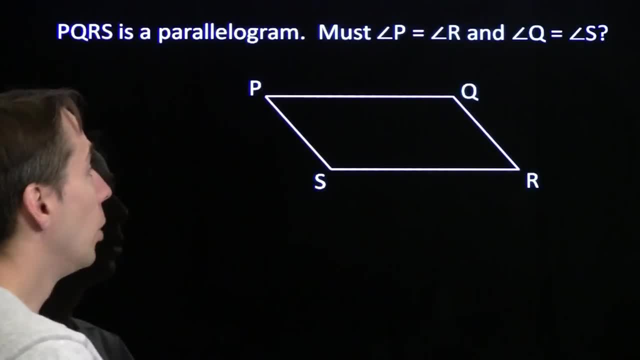 equal. These two opposite angles are always equal. We aren't given any angle measures here. so if we can prove it here- and that shows it's true always, How are we going to do this? I'm going to start off by calling this angle. 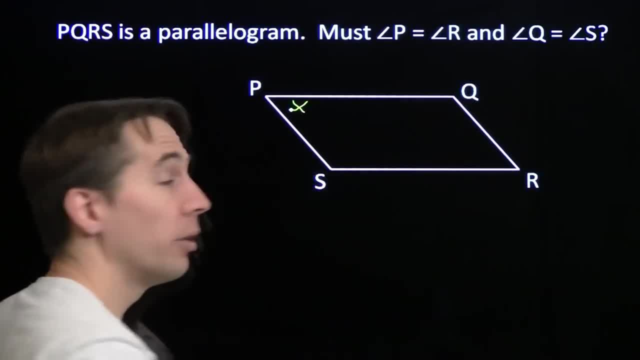 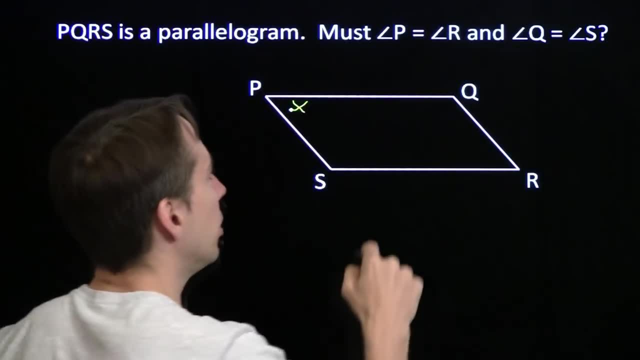 measure x. Now it's a parallelogram, so P, S and Q are. they're parallel. So this angle over here has to add: with this angle, P plus Q has to add up to 180 degrees, So this angle. 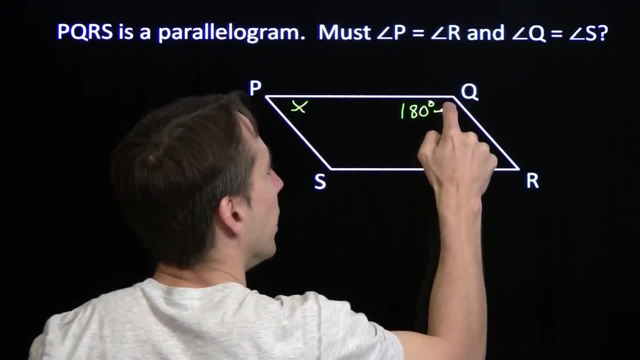 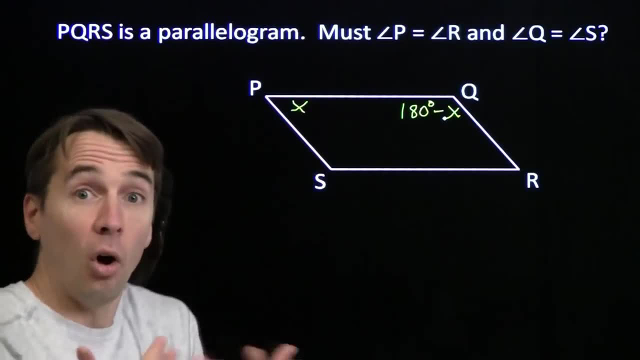 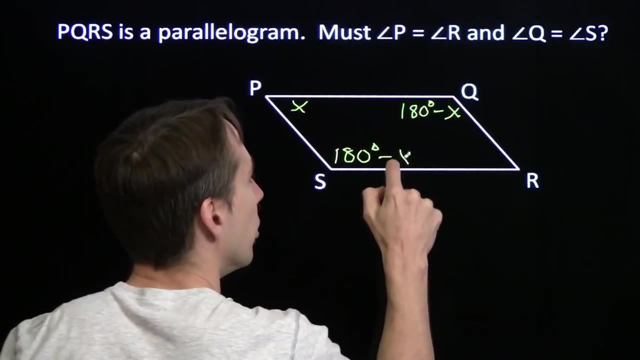 over here has to be 180 degrees minus x. Well, P, Q and S are parallel, So angle P and angle S also have to add up to be 180 degrees. So angle S is also 180 degrees minus x. So sure enough, we see, Q equals angle S. Check. 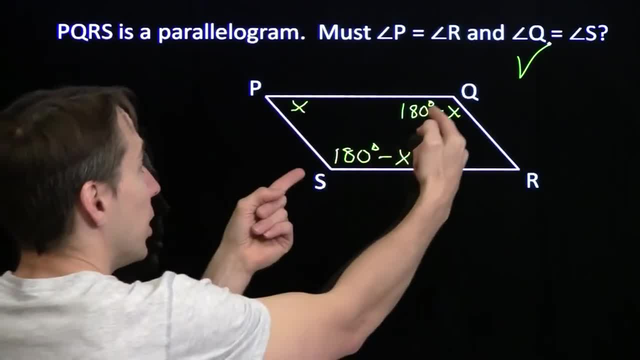 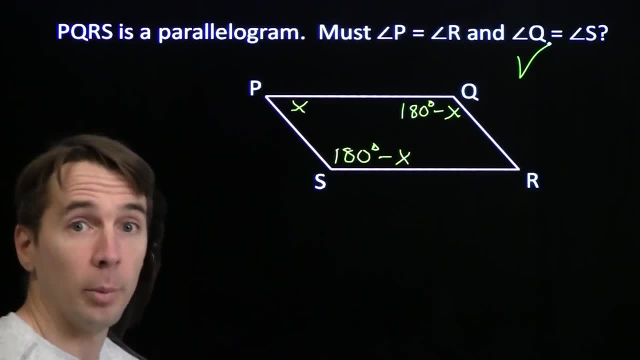 We know that's for sure. those two always have to be equal. We can say that by just noting that Q and S, each of them, has to be supplementary to angle P. They're supplementary to the same angle. they have to be congruent. What about angle R here? Well, angle R we. 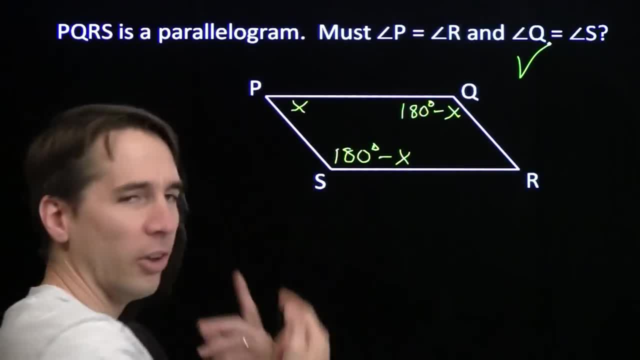 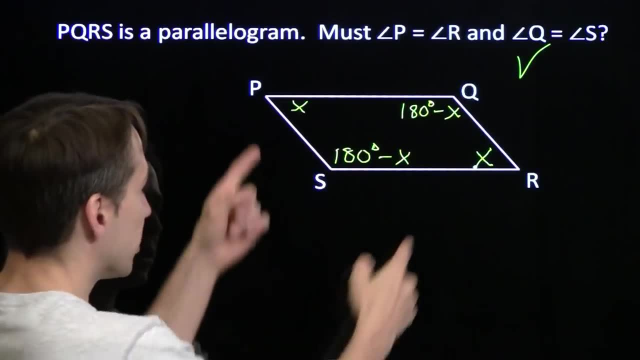 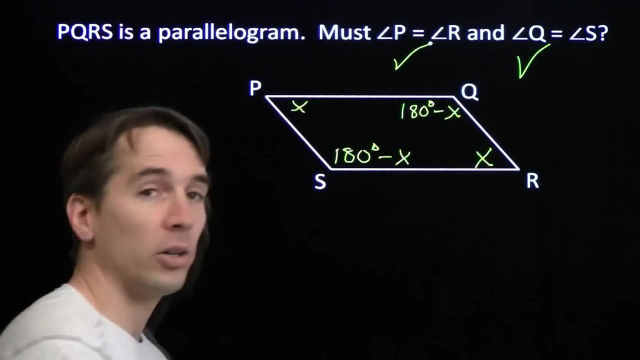 got QR is parallel to PS. so angle R plus angle S has to be 180 degrees, And that of course means angle R is X. So we've got angle P equals angle R as well. So the opposite angles of a parallelogram are always congruent. So, coming back here, knowing that fact once, 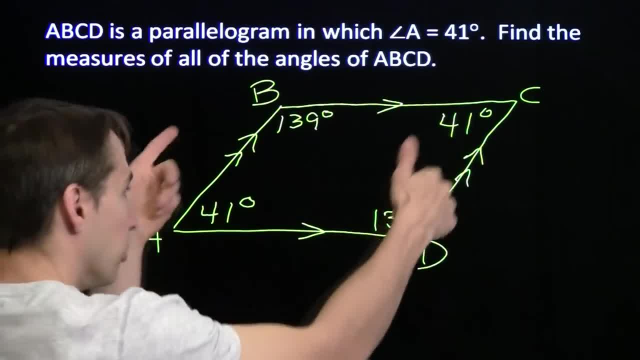 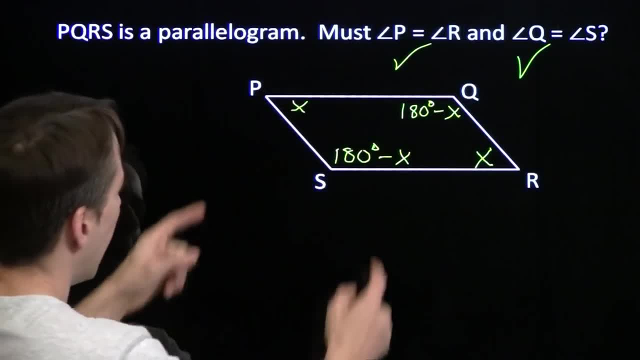 we had this 41, we could immediately write that 41 over there. Then we can use our parallel lines to find that this is 139, and we immediately know that that one's 139 as well. So opposite angles of a parallelogram are equal. Opposite angles of a parallelogram. 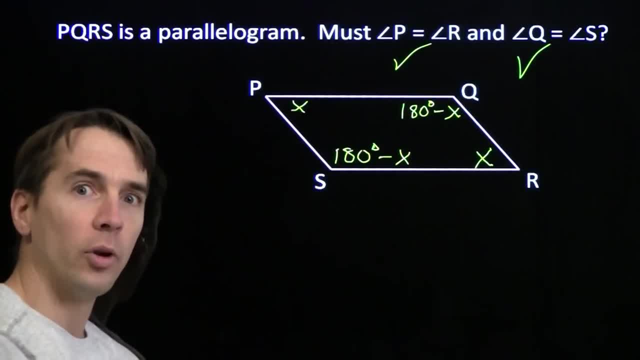 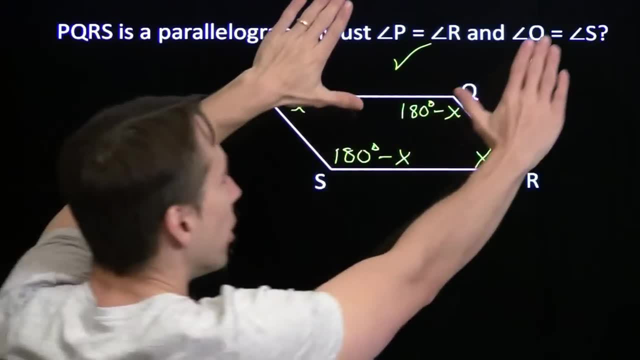 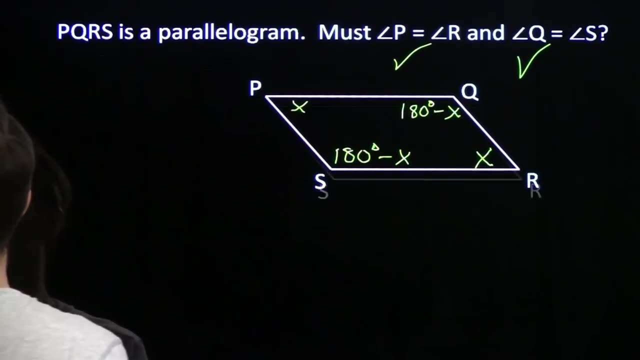 are equal. What if we have the opposite angles in a quadrilateral are equal. Does that mean the quadrilateral has to be a parallelogram? Can we run this straight backwards and start here Opposite angles are equal and end here? Quadrilateral is a parallelogram. Let's check that out. Suppose we start off and all we 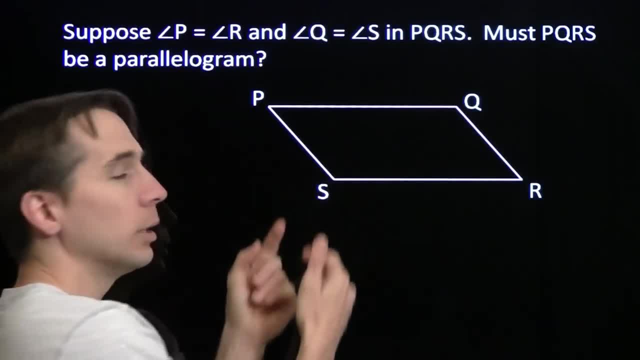 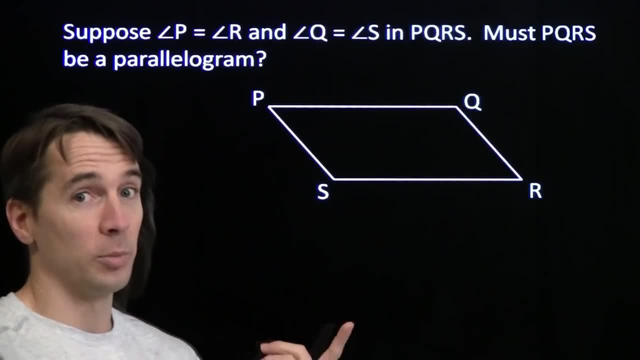 know is that P equals R and Q equals S, And we want to determine whether or not this is a parallelogram. Sure, looks like a parallelogram, but you know I can trick you with my drawings, So we're going to have to prove it here. P equals R. Once again, we'll break out some. 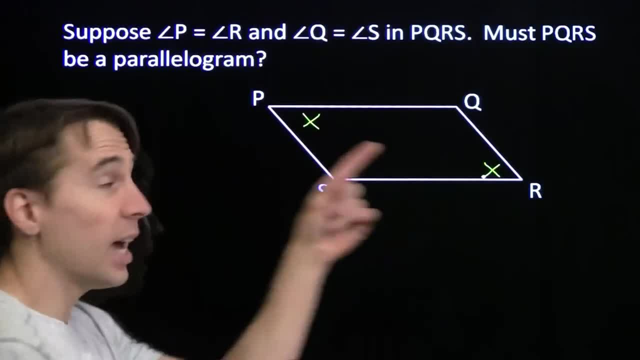 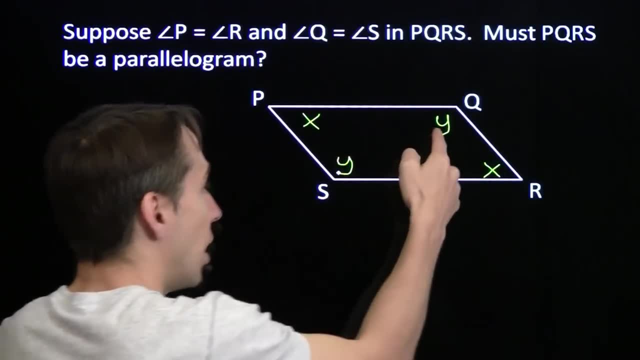 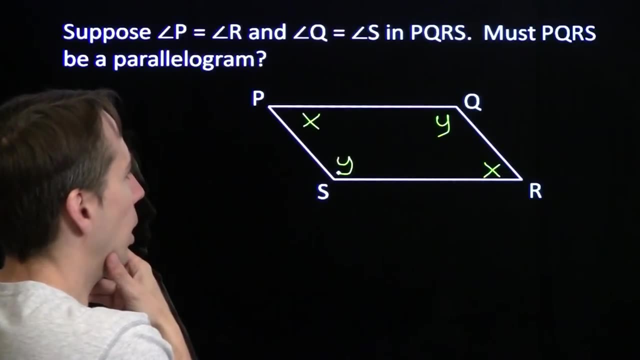 variables. Call each of these X because they're equal, and Q and S are equal as well, And pick another variable, Y. Now we can't say that this is 180 minus X, because we don't know that these sides are parallel. yet That's what we're trying to prove. Now what Well. 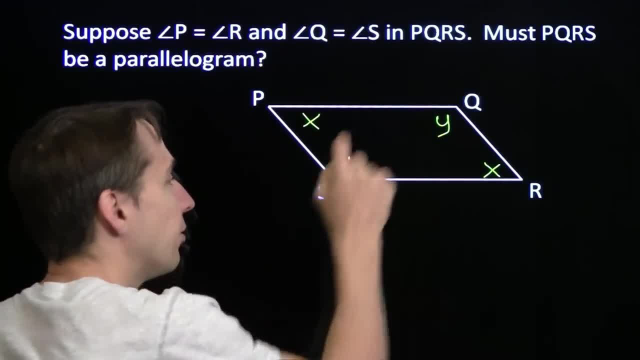 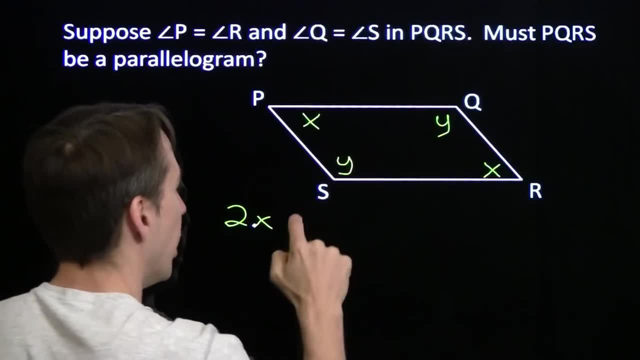 we've got all four angles here of a quadrilateral. We know that they have to add up to 360 degrees. So when we add all four of these we'll get 2X and we'll have 2Y And that has to all. 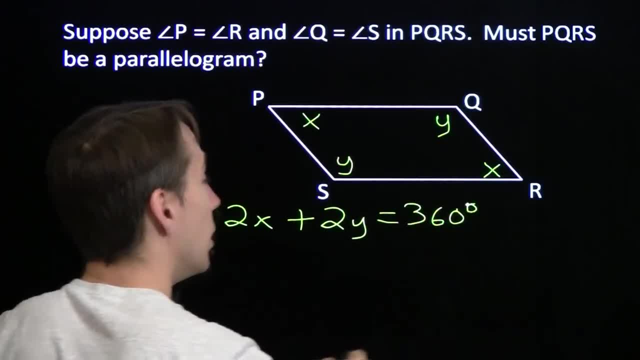 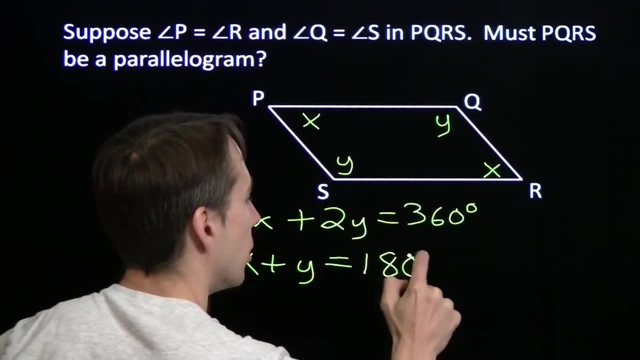 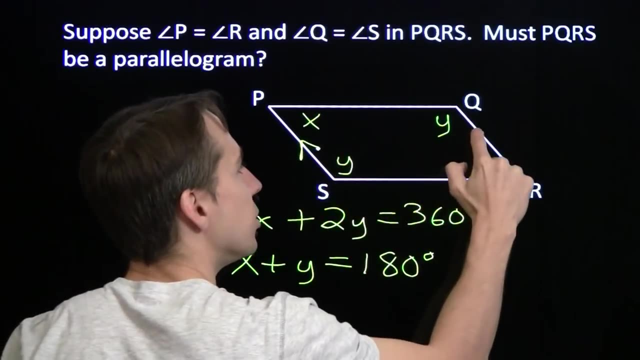 add up to 360 degrees. So we're going to divide everything by 2, and we'll get: X plus Y is 180 degrees. Well, X plus Y is 180 degrees. If this plus this is 180 degrees, that means that these two 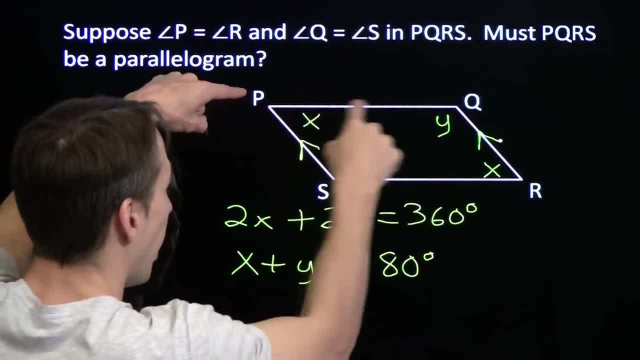 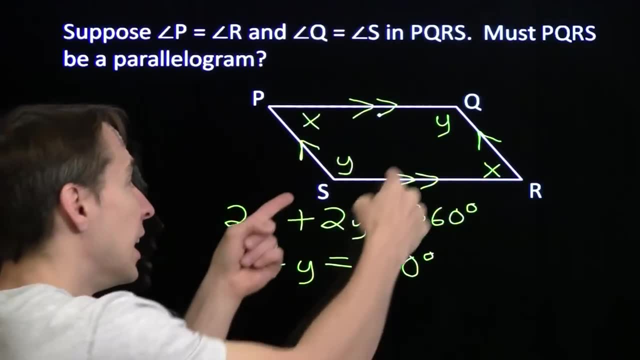 are parallel. And the same thing here. This X plus this Y is 180 degrees. That means that these two sides are parallel. So, sure enough, this street does run the other direction If the opposite angles of a quadrilateral, each pair of opposite angles, is congruent. 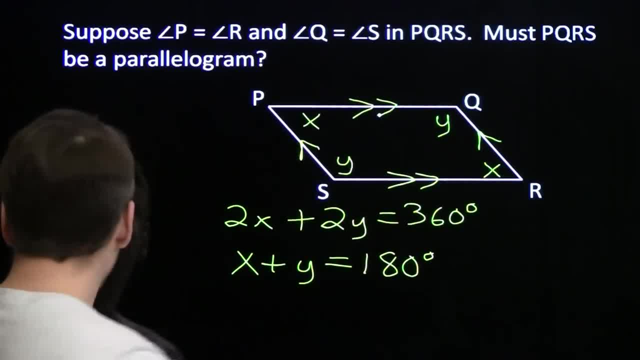 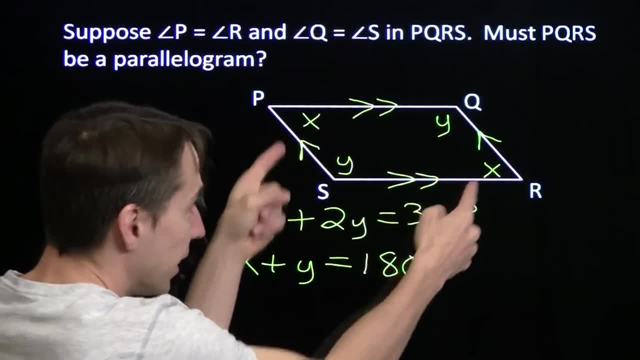 then we know that the quadrilateral is a parallelogram. So quick recap: Opposite angles of a parallelogram are congruent and we can go backwards. If we find out that the opposite angles of a quadrilateral are congruent, then we know: that the quadrilateral is a parallelogram. 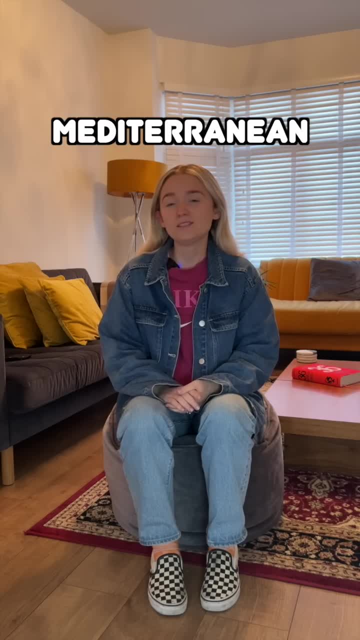 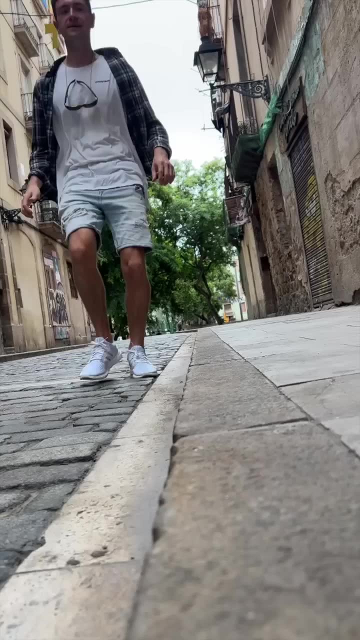 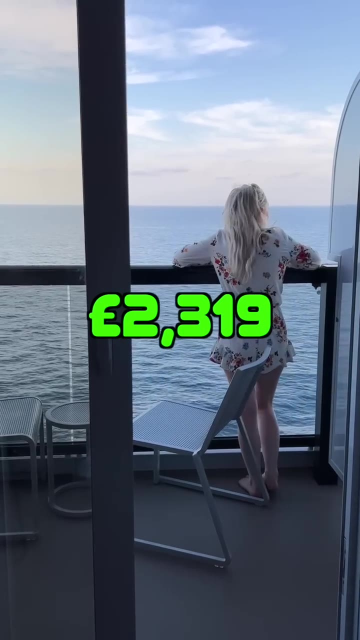 Are cruises expensive? If you go on a seven-day Mediterranean cruise visiting five cities in three countries, would it just be cheaper to travel to these places on your own? Let's break it down: A seven-day Virgin Voyages Mediterranean cruise costs £2319 for two people. 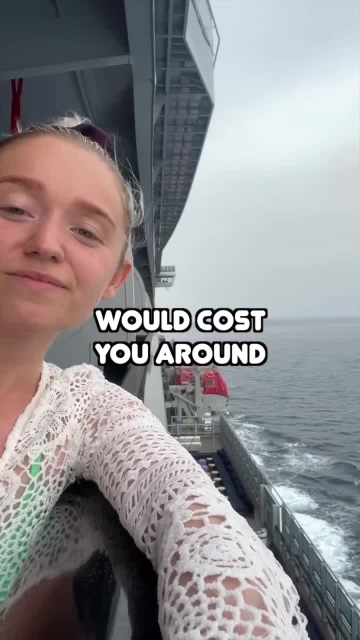 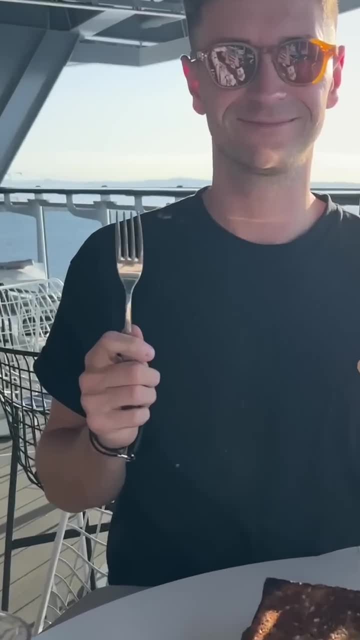 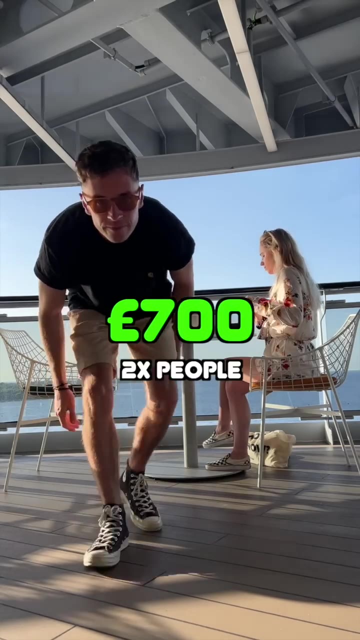 Seven nights hotel accommodation across five cities will cost you around £843.. All food and drink are included within the price of the cruise. So let's say you fork out £10 on breakfast, £15 on lunch and £25 on dinner For two people across seven days it comes to £700.